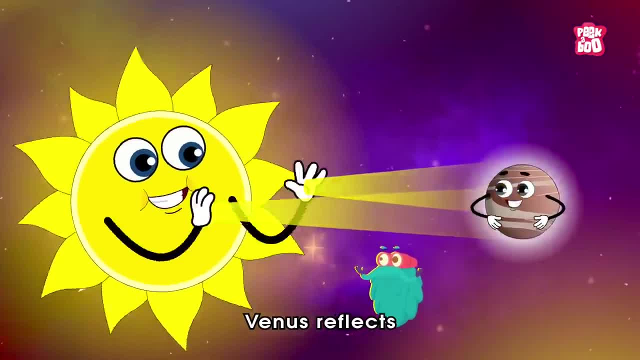 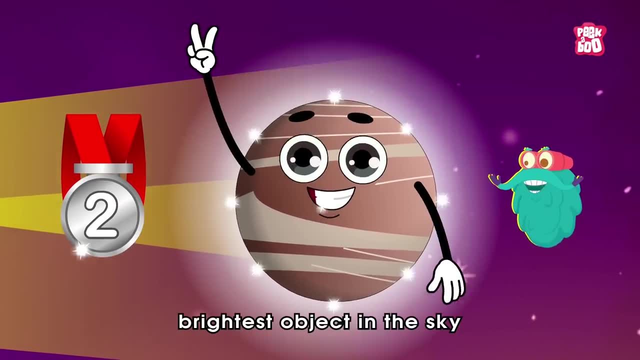 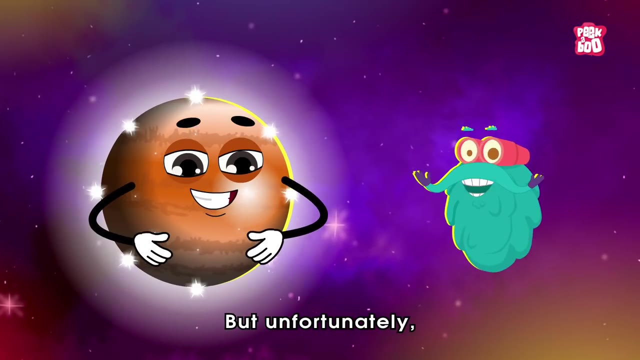 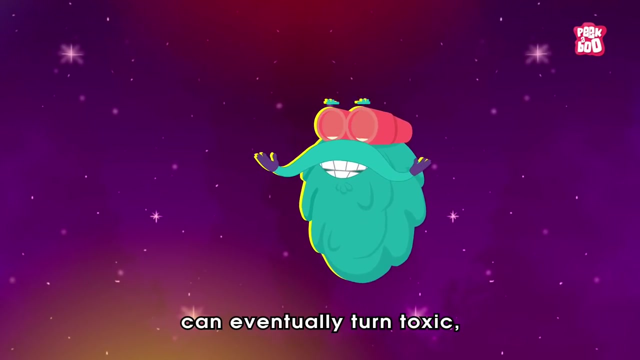 Not only that, Venus reflects 70% of all the sunlight it receives, and that is why it is the second brightest object in the sky, after the Moon and the Sun. But unfortunately, not everything that shines is gold, And what seems like love at first sight can eventually turn toxic. 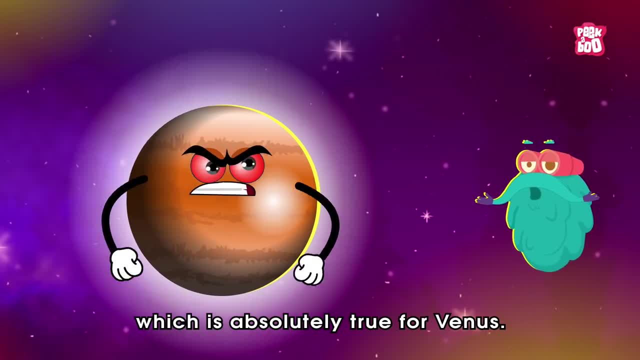 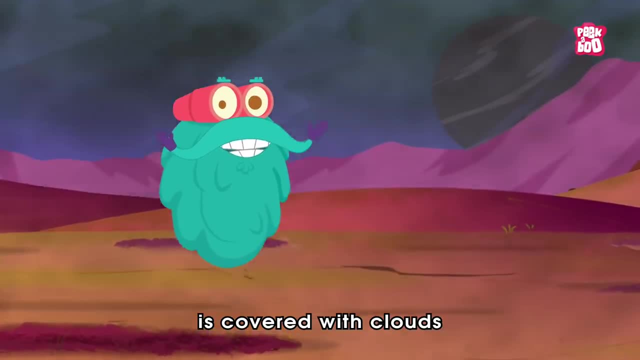 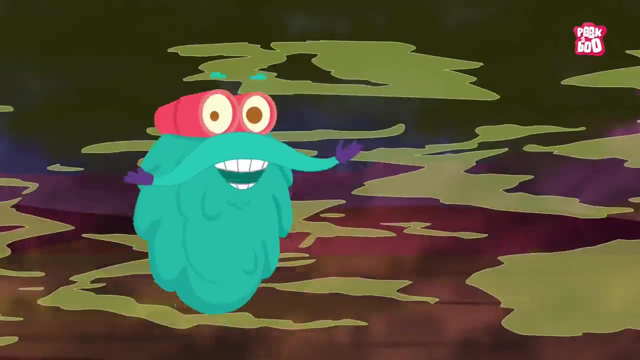 Which is absolutely true for Venus. Yes, that's because Venus's entire surface is covered with clouds made of poisonous sulfur dioxide, giving us enough reasons not to step on the planet. And if we need to know what happens if we try to step on Venus, 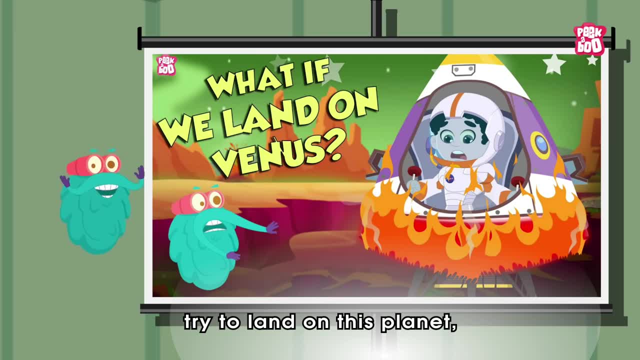 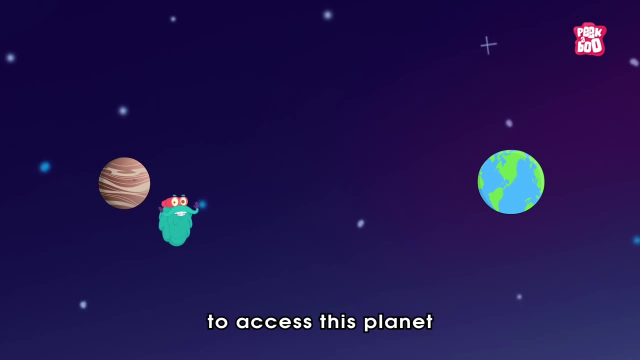 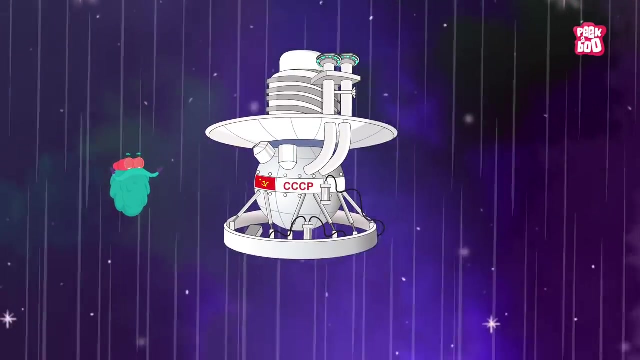 Then please check out our video. What if we landed on Venus? The link is in the description below, But it does not mean that no attempt was made to access this planet, as the first spacecraft to set mechanical feet on another planet landed on Venus. 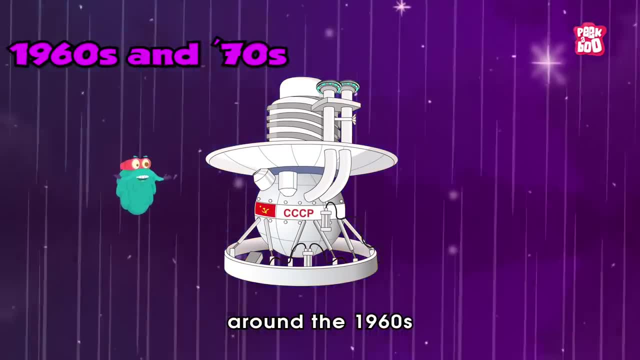 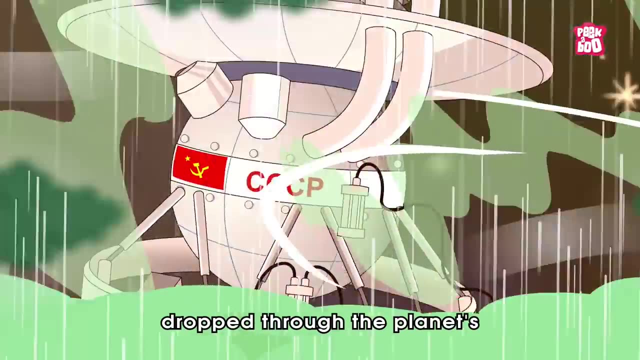 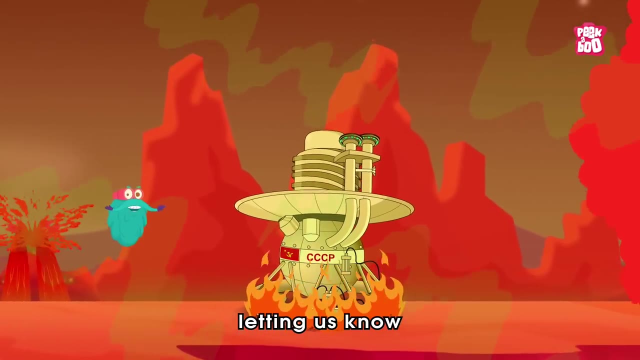 Yes, around the 1960s and 70s, The former Soviet Union's Venera probes, dropped through the planet's unbearable atmosphere, managed to send back essential data on Earth, letting us know that Venus is like a massive pressure cooker. That's true, my friends. 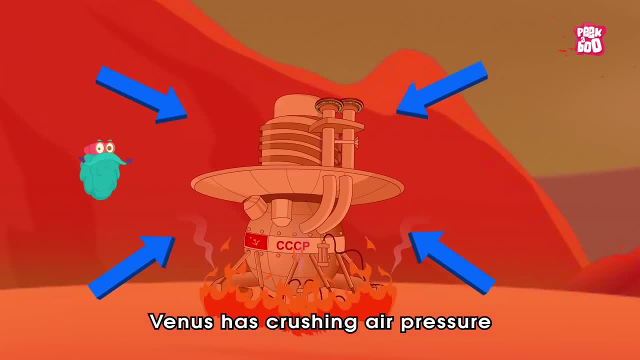 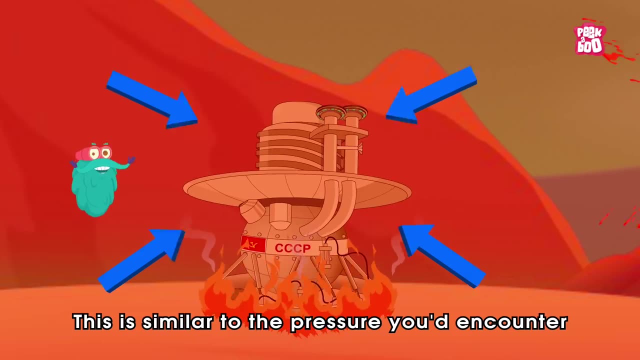 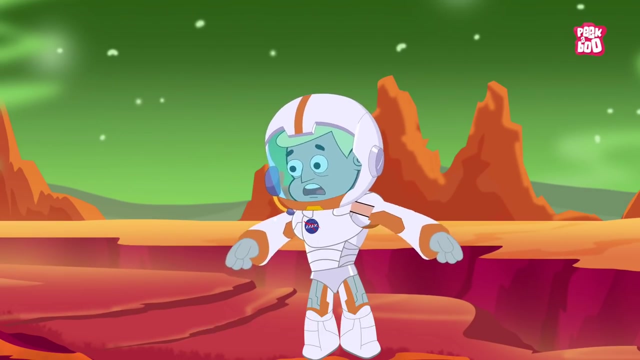 Venus has crushing air pressure at its surface which is more than 90 times that of Earth. This is similar to the pressure you'd encounter a mile below the ocean on Earth. This pressure is so intense that a human standing on its surface would be crushed. 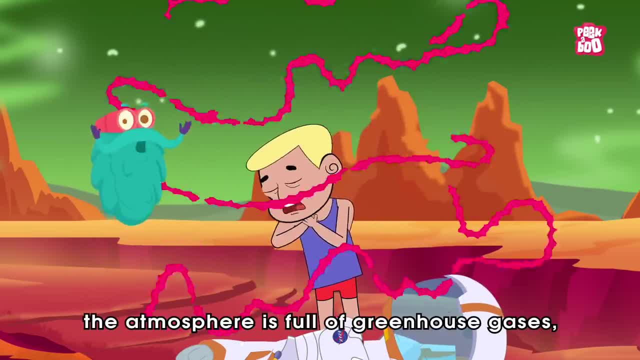 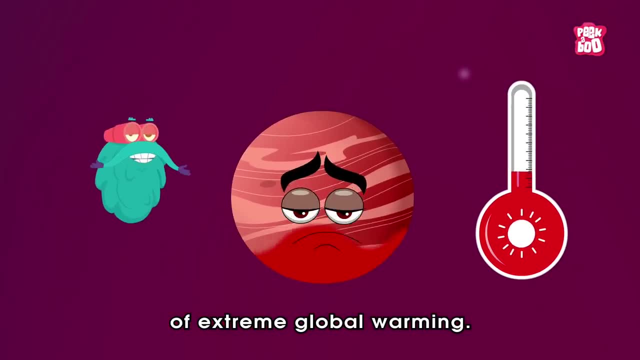 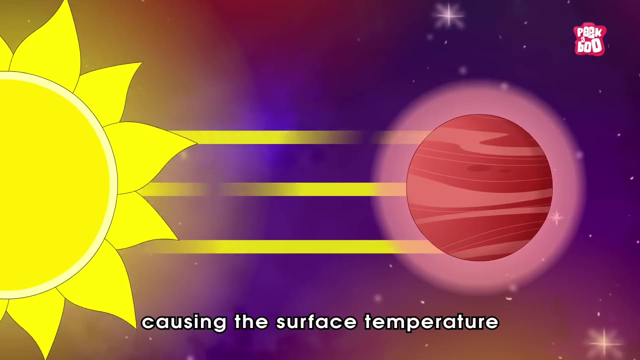 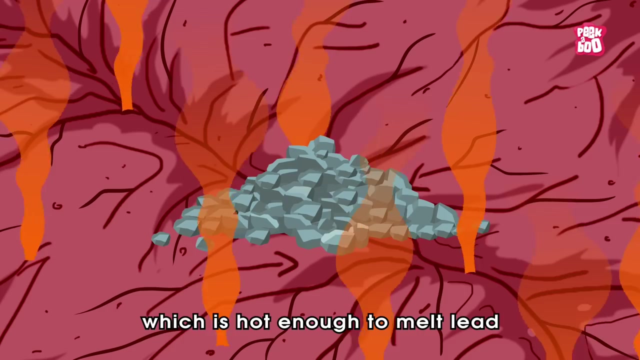 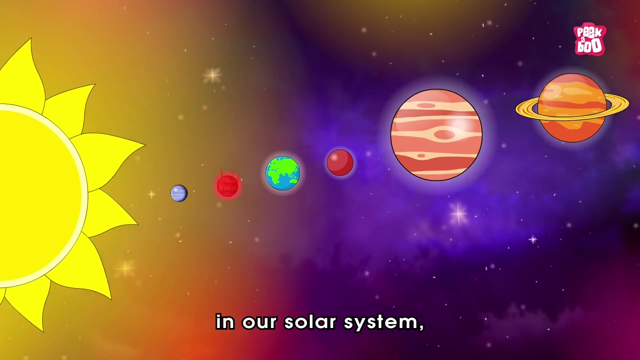 And, on top of that, the atmosphere is full of greenhouse gases, mainly carbon dioxide, leading to the issue of extreme global warming. The atmospheric layer travels through the atmosphere. That layer traps the Sun's heat, causing the surface temperature to go over 880 degrees Fahrenheit, which is hot enough to melt lead, and declaring Venus the hottest planet in our solar system, despite Mercury being closest to the Sun.